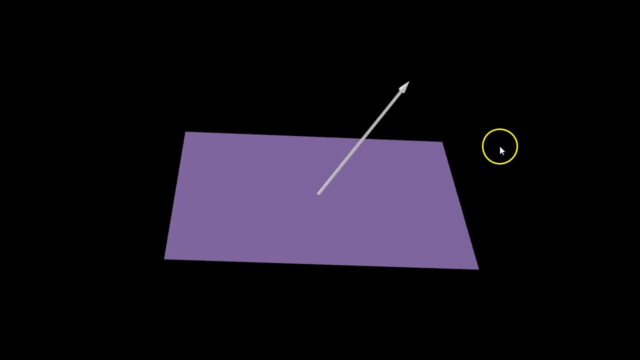 here. I might have a vector here, this white vector, and I want to project it onto that purple plane And there's a there's a pretty straightforward way of doing that, if indeed I have an orthonormal basis for that purple plane. 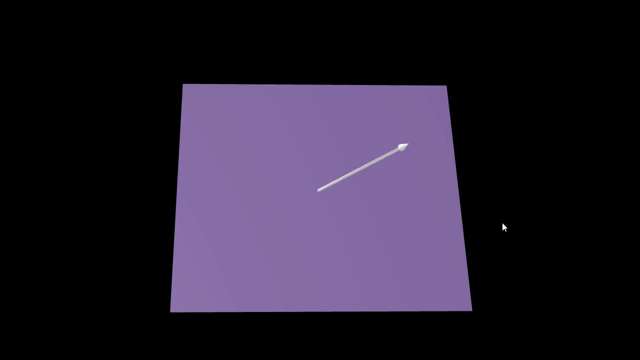 it just involves doing a couple projections onto the basis vectors And that, of course, looks like this: the projection vector would be this and it's perpendicular component would be this: and the point is, how do I get these two blue vectors from that white one? And again, if I have an orthonormal basis for 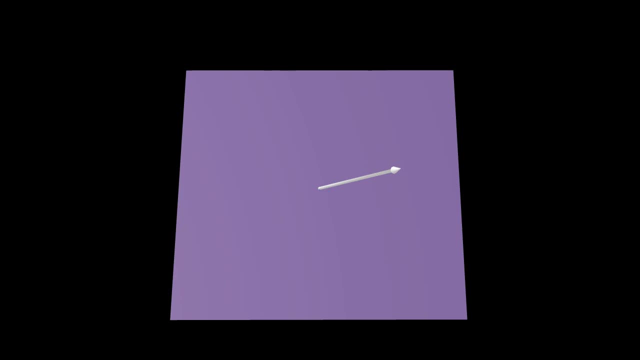 the purple plane. there's a way of doing that So, but the problem is that it might not be totally obvious how to get the orthonormal basis, but it might be rather straightforward to get any old basis for this purple plane I might have. 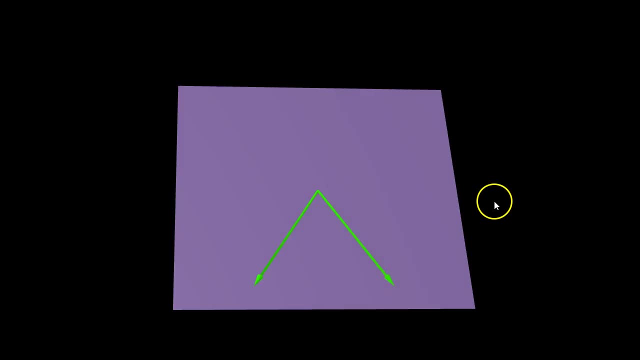 already been, given that maybe that's how the plane was described or maybe, if I had an equation for the plane, I could do a little arithmetic and try to find a couple of vectors, which I might not be able to do. So I'm going to go ahead and 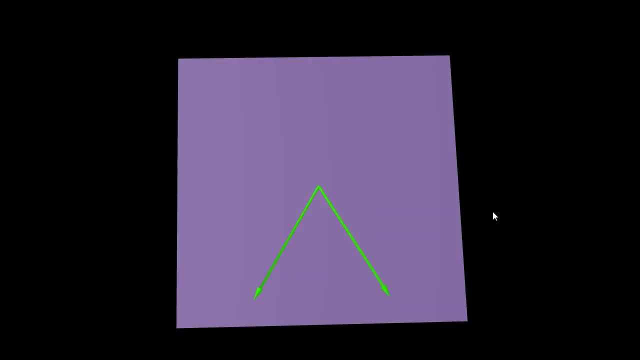 do a little arithmetic and try to find a couple of vectors which are a spanning set for that plane. but you can see if I come up with, say, two basis vectors, say these two green ones. they're not orthogonal to each other and they're probably not even of length one. 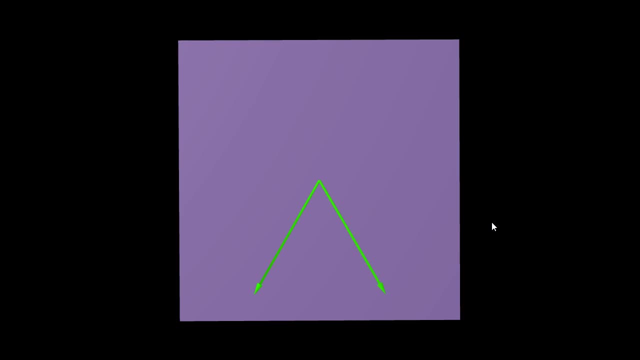 so they're not an orthonormal basis, but they are a basis. and the question is: can I work with that somehow? Can I kind of coax those into being an orthonormal basis by altering them in some way? So there's a way of doing that. but let me 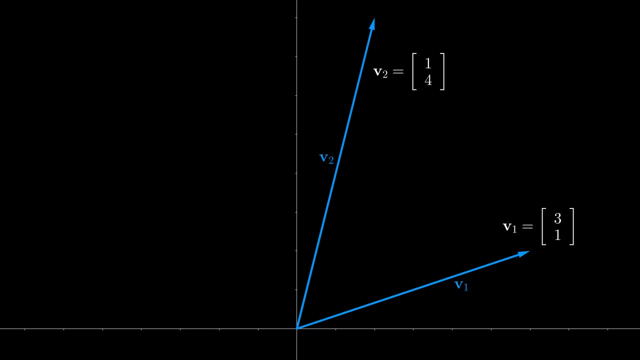 show you how that works in two dimensions here. It's easier to see what's happening if we do this in 2D. So let's move here to 2D. I have two vectors here, V1 and V2.. Those are indeed a basis. 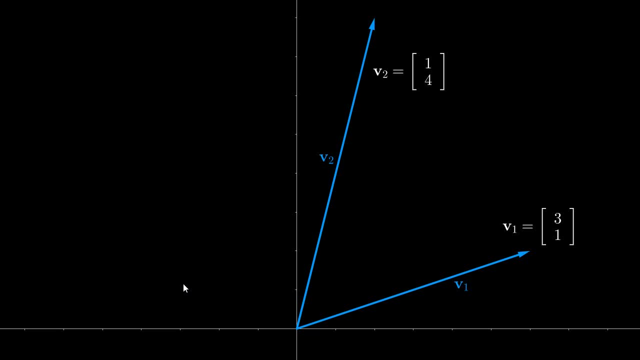 for R2.. Of course we already have an obvious orthonormal basis for R2.. That's E1 and E2, 1, 0, and 0, 1.. But the point is, I want to think about that more general situation where I have a 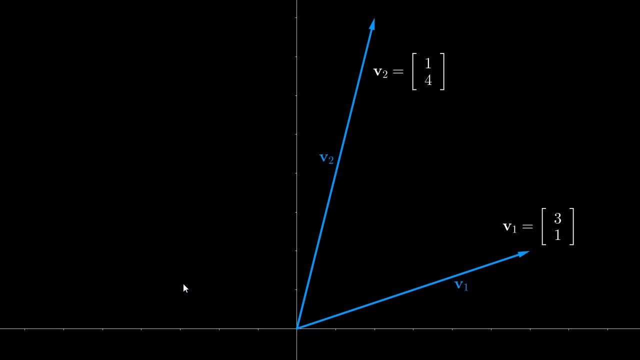 basis already. I want to try to tweak it somehow and kind of convert it or get an orthonormal basis from that. So let's start with having V1 and V2 here and see if I can kind of alter them in some way to get an orthonormal basis. So V1 and V2 are the vectors as shown. Those are not of length. 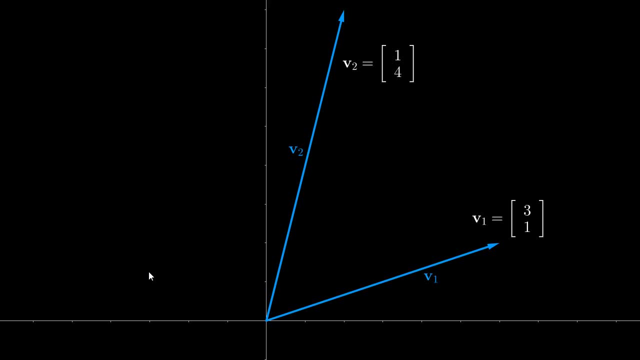 1. V1 has length. what is that? square root of 10,, I think, And they're not even orthogonal to each other either. So here's the process. Now let me get rid of the labels here. I don't really want. 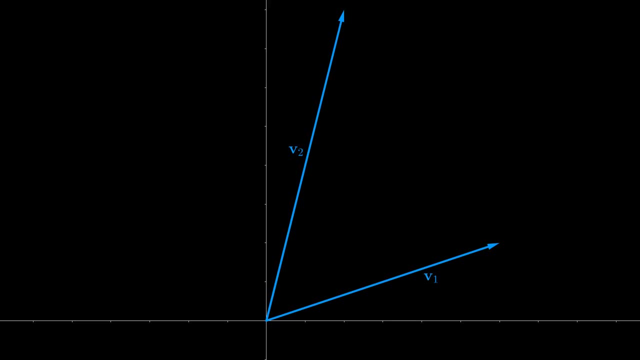 to think about the numbers so much. I want to just think about the geometry of this And let's go through the idea. What we're going to do is we're going to keep V1. This vector V1, we're going to hang. 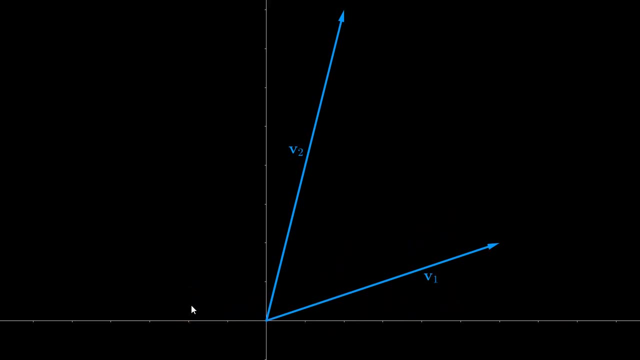 to that one. we're going to keep that in our basis, except it's not of length 1, so I have to fix that its length is square root of 10 right now, or something like that. so what I'm going to do is I'm going to shorten it. I'm going to 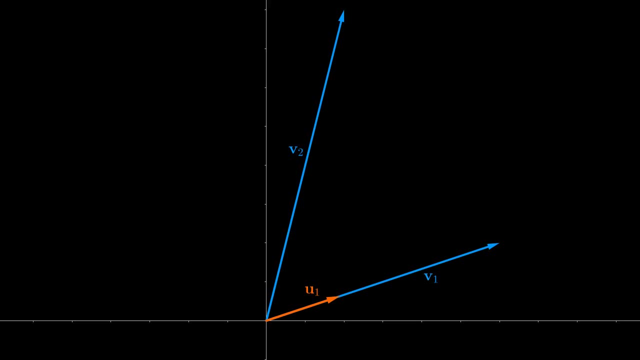 shorten it down to a unit vector and you would say you're normalizing the vector when you do that. so you know how to do that. you multiply by 1 over the magnitude, and that would convert it to this orange vector here. so then I'll let 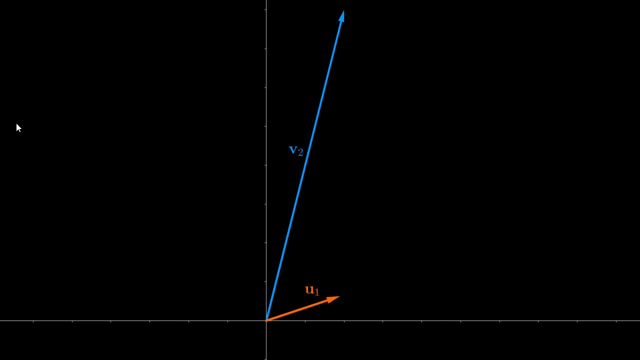 me get rid of v1, so I'm replacing it with u1, so u1 is just a shortened version of v1. and then what we're going to do is we're going to take v2 and we're going to extract out of that something which is orthogonal to u1, and 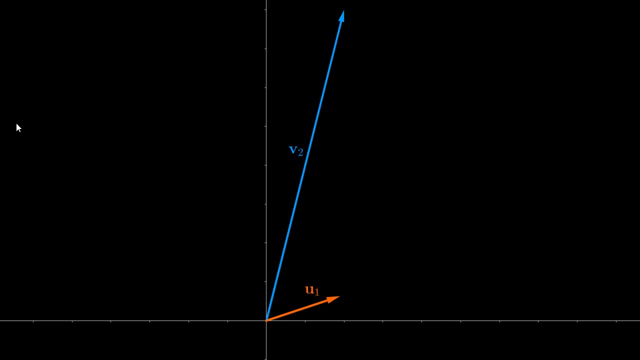 that'll be our other basis vector. what's kind of important right now about v2 is that it's not parallel to u1. it couldn't be, because v1 and v2 are a basis for r2, so v2 is definitely not parallel to u1. that means that v2 has a parallel. 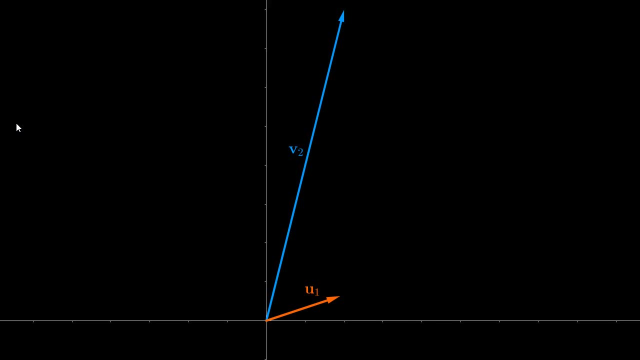 component to u1 and a perpendicular component to u1, and that means that v2 has a perpendicular component to v1- excuse me- to u1, which is nonzero. so you know how to do this. I'm going to project v2 down onto the u1 vector. I. 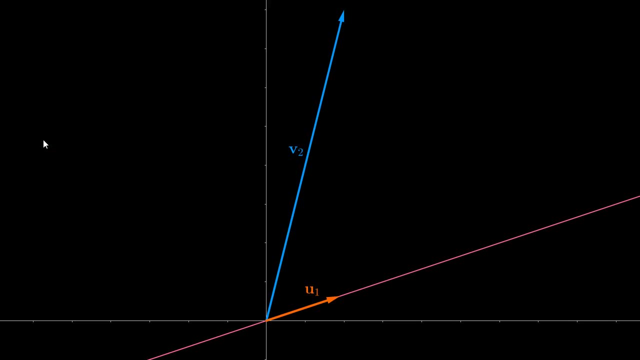 guess what I really mean when I say that, when we say we're projecting a vector onto another, is we're projecting the blue vector down onto the space spanned by u1, this line here. so that would look something like this: we drop a perpendicular down and this is geometrically what's happening. 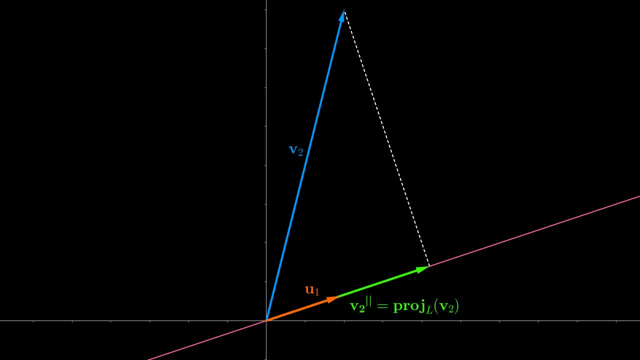 and then the projection vector looks like this. this green vector here is the projection of the v2 onto the line spanned by u1, and then the perpendicular component of that is obtained by a subtraction. right, we're just going to take v2 and subtract off its perpendicular component, and then we have. 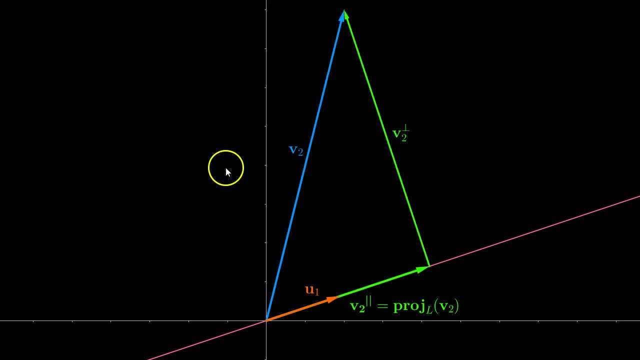 v2 perpendicular. there- I don't know if I said that right- we're going to come subtract a parallel component from v2 to get the perpendicular component of v2 and that's it. this is going to be our vector that we're going to use for the. 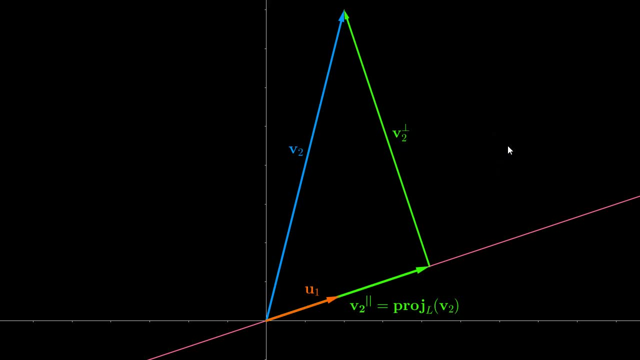 basis v2 perpendicular- let me draw that, though, over coming out of the origin, because that might be a better place to see it, and hide some of these other components here- and u1 and v2 perpendicular are now indeed orthogonal to each other, and they serve as a basis for r2. there's only one last thing to do. 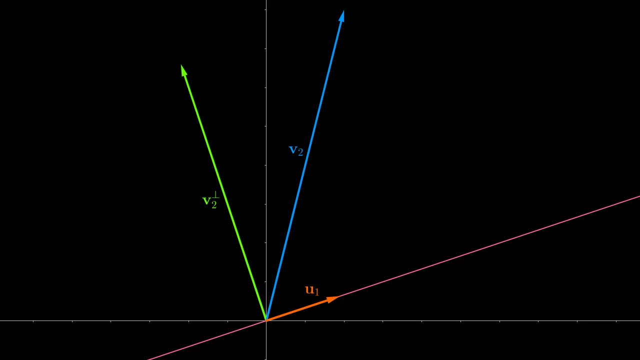 v2- perpendicular- is not of length 1, and it's an easy conversion to normalize that. you divide by its length and you get a vector which is indeed of length 1, and that would give us a vector we can call u2. so now u1 and u2 are both of length 1 and they're perpendicular to each other. so 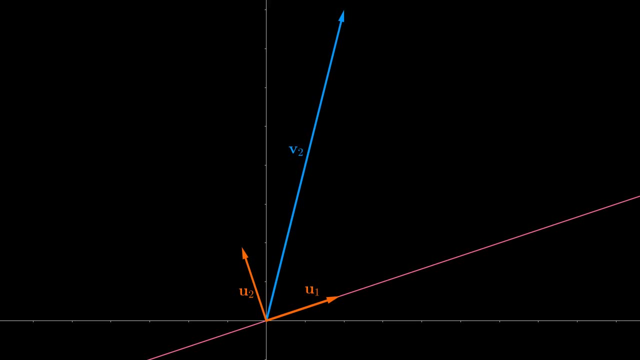 they are an orthonormal basis for r2. and again, remember how we did that. we started with two vectors, v1 and v2. let me hide this L here. we started with v1 and v2 and we kind of coaxed them into giving us an. 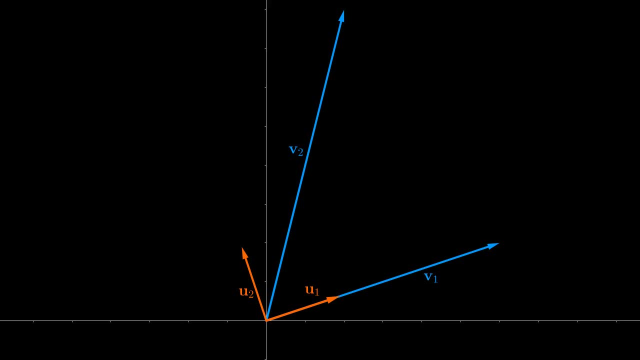 orthonormal basis for r2. we kept v1, we just shortened it down, and then we took the part of v2 which was perpendicular to that first u1, and that's called the Gram-Schmidt orthogonalization process for getting an orthonormal basis. 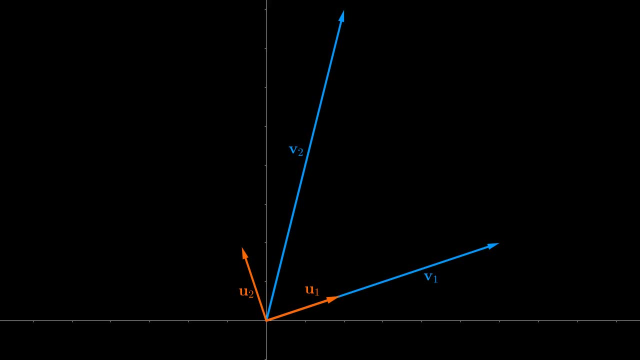 starting from some other basis that you have. so now remember that these vectors were very specific. v1, v2 had specific components to them. maybe you can kind of go back watch the video again and see if you can actually work out the numbers here. what exactly are u1 and u2 there as vectors? follow through with the. 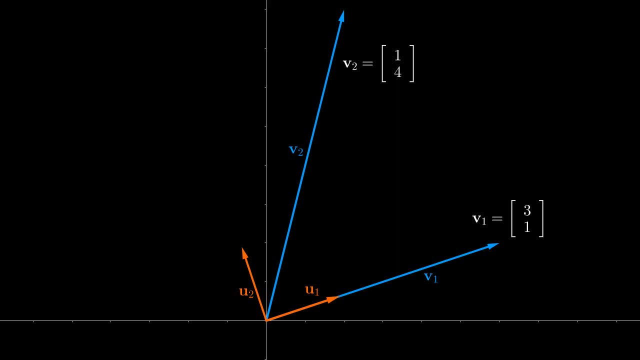 projections and subtraction and all that and see what you get. 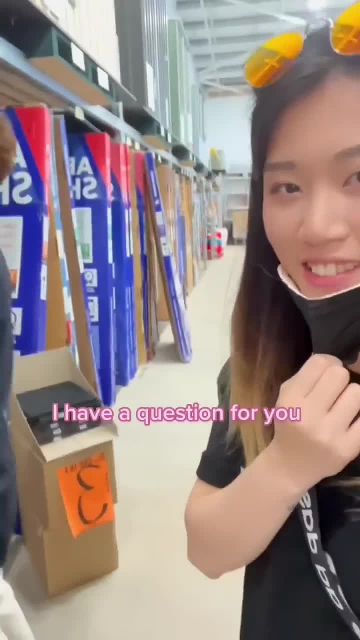 Testing my boyfriend IQ. I have a question for you. What is it? If you get it right, I'll pay for everything. Okay, sounds like a deal for me. Okay, so from 1 to 10, how many 8s are there?